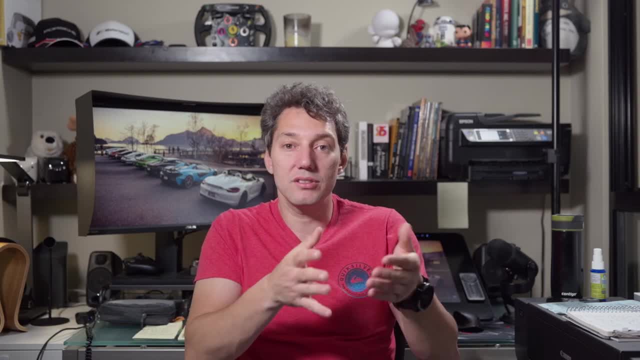 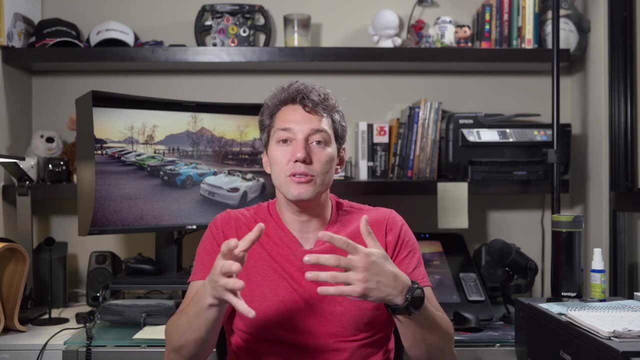 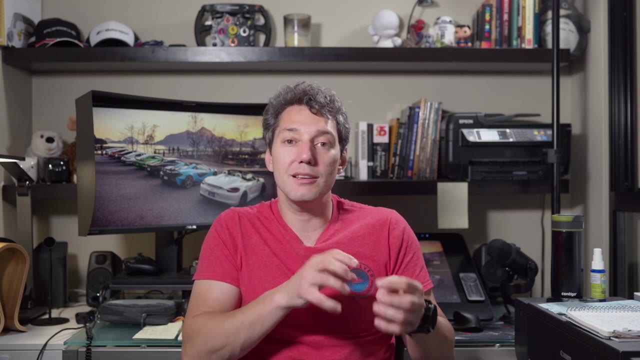 that is actually affecting how the light is bounced back into our eyes. you will see that, while the pigments stay consistent, if we move around, we don't see color changing. In that case, in the case of this specific butterfly or other objects that are similarly structured, 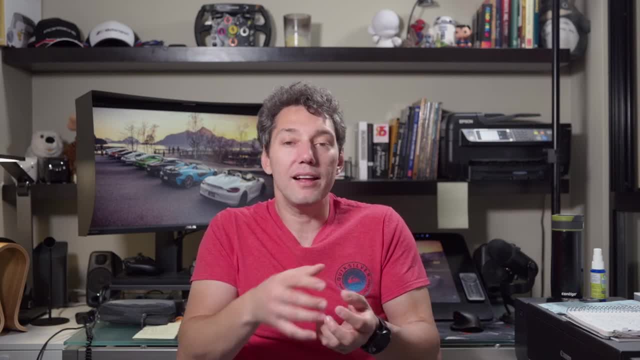 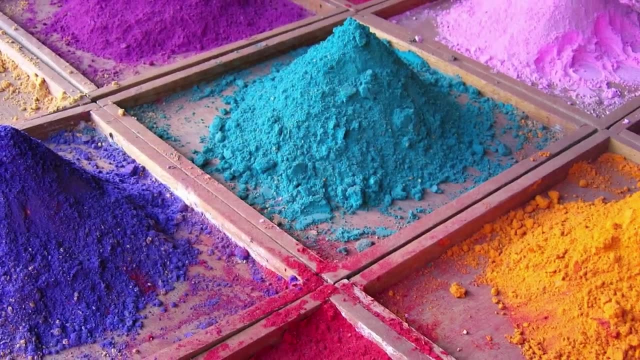 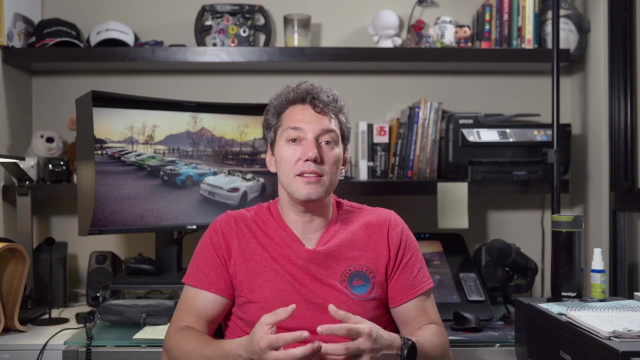 when you move around, there are differences in the way the light is bounced to our eyes. In nature there are all sorts of pigments, and pigments is basically what was used originally to create colors that then the artist would use. But the real pigments or the real colors have only 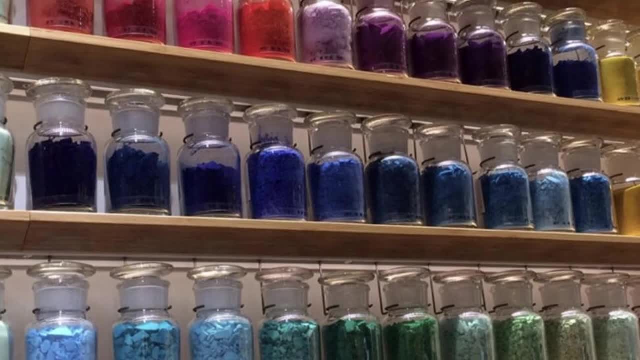 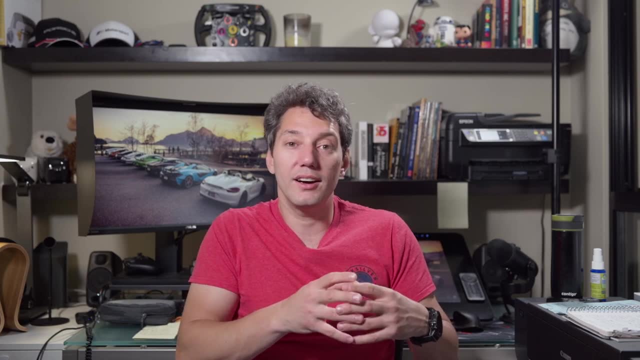 been developed in the 1800th century. Before that there were a lot of scammers that would sell artists colors that would discolor quickly or maybe would also tint with the canvas. They would react to the canvas and so it was a little bit of a hit and 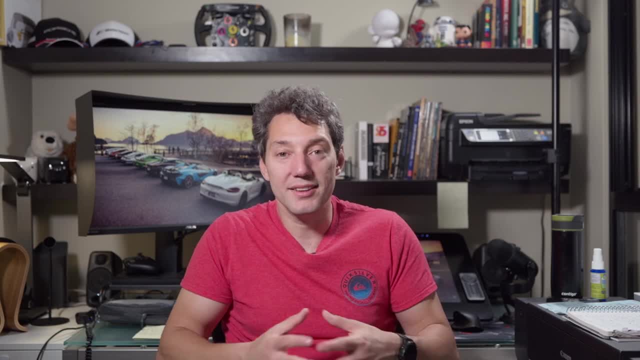 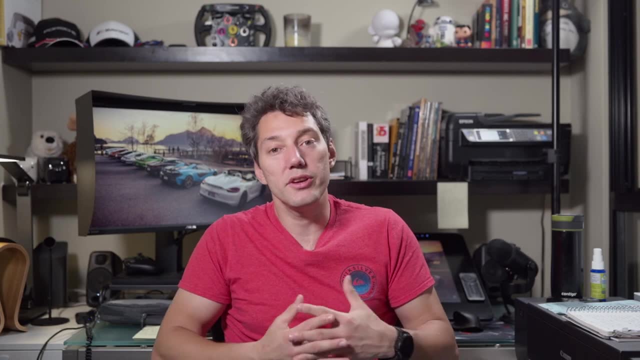 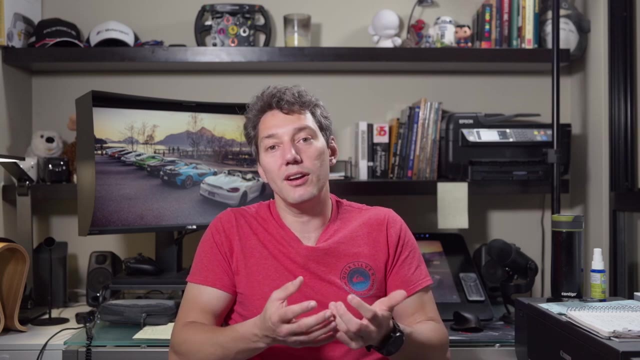 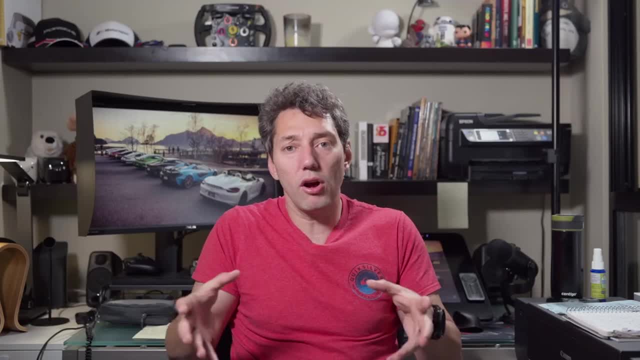 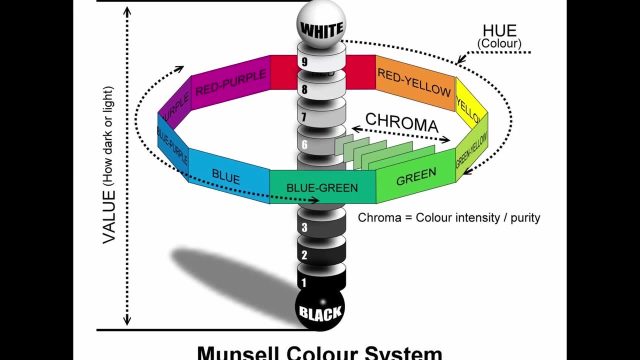 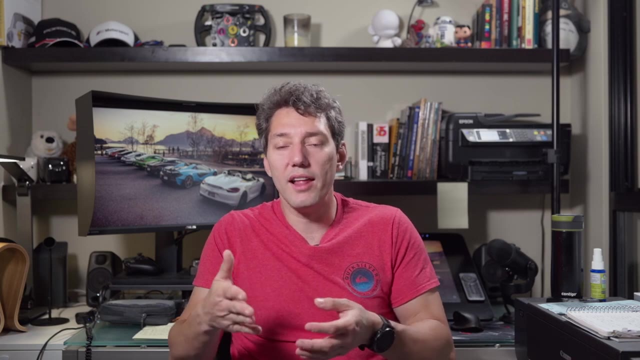 the color theory, But it was Munzel that actually picked this color that Newton discovered and put them along the color wheel, which is probably the most used tool for an artist today. He also associated the colors with notes, with musical notes, starting from the red and the C, and then 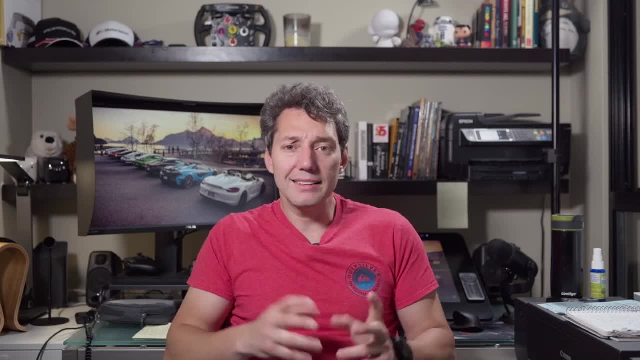 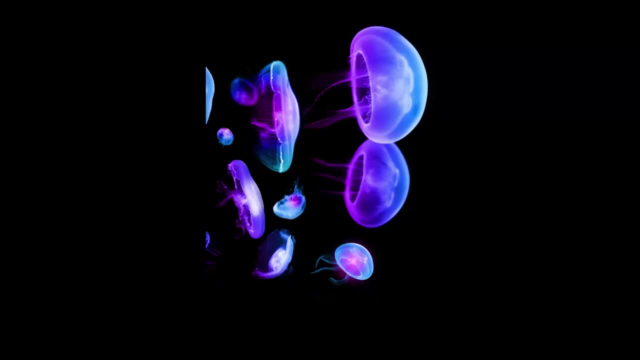 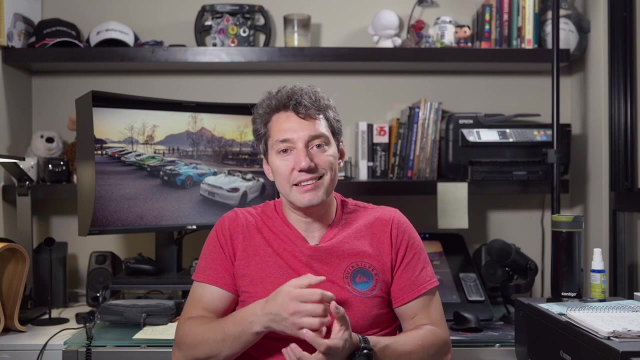 moving forward according to the order of the notes. There are then other categories of objects that have very specific features, like, for example, luminescent or phosphorescent or fluorescent- objects that, basically, are capable of either emitting light or absorbing light and releasing it slowly so that they can conserve effectively. 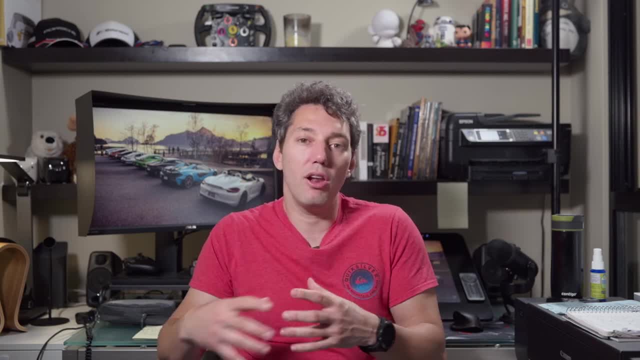 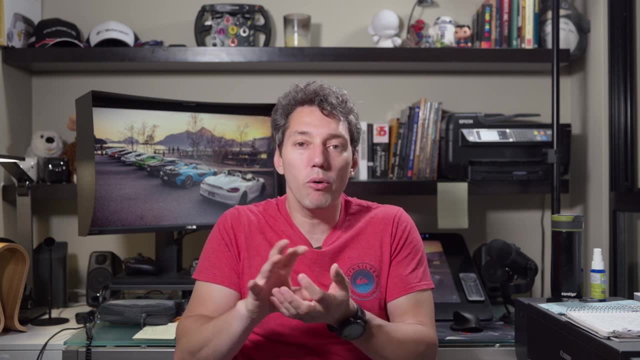 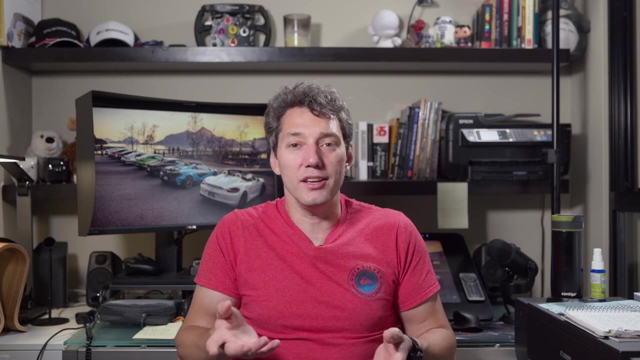 these photons, this energy inside their bodies for a longer period of time, and the light, instead of being reflected all at once, is basically staying in the body and then slowly, slowly, slowly released. so if you understand now what pigments are, it might be true that we are what we eat. 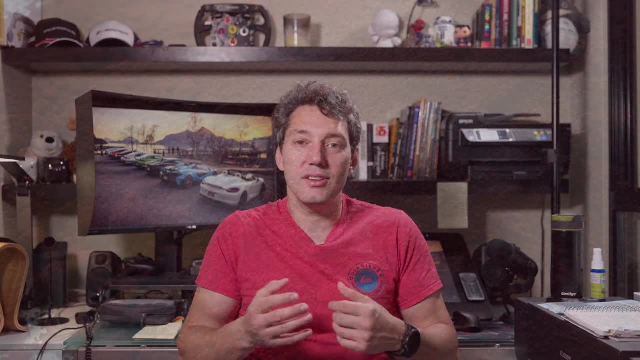 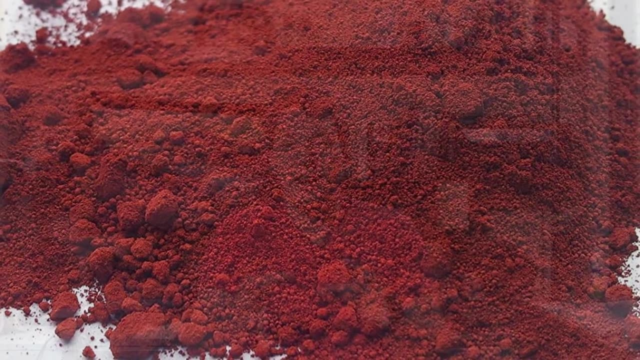 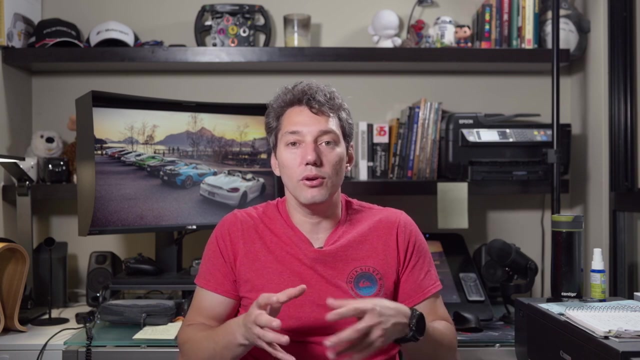 and, for example, even mars is red because there is iron oxide, which is the same substance that is also in our blood and has this reddish color. now, some pigments in nature are more rare than others and, in particular, if you look around you like, you won't see many objects in. 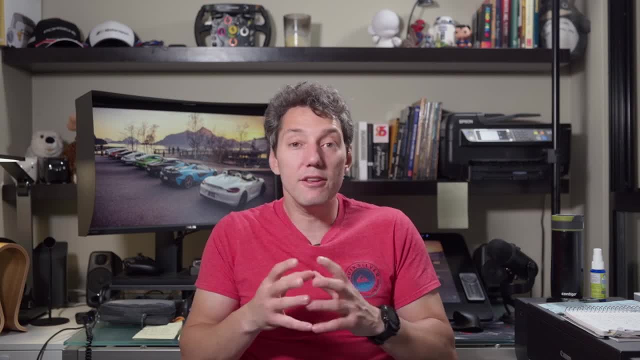 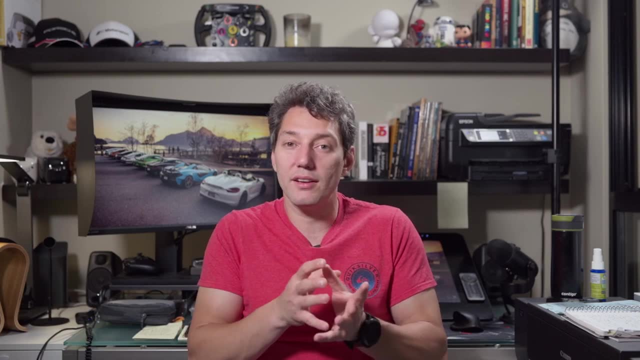 nature that are blue, and there are very few animals as well that are blue, and one is the butterfly we talked about. that is not really a pigment. it's not really blue because it's a pigmented blue, but it's because of their structure that reflects the 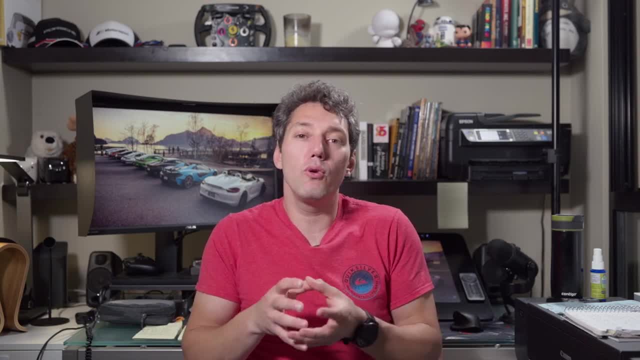 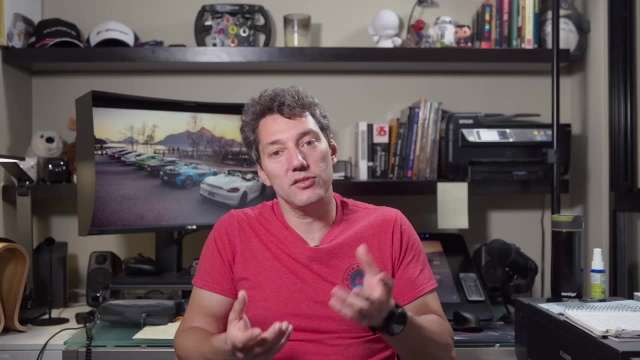 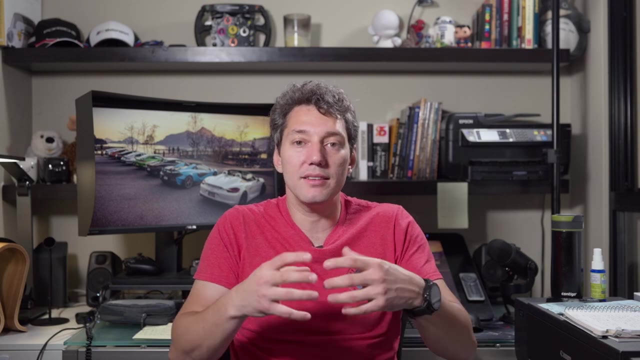 light that way. there are some animals, though, that have this blue pigment, like, for example, the blue poison dark frog. today, though, we don't really use these pigments as much as we used to, because we have synthetic pigments, synthetic colors, which are basically made of multiple elements and 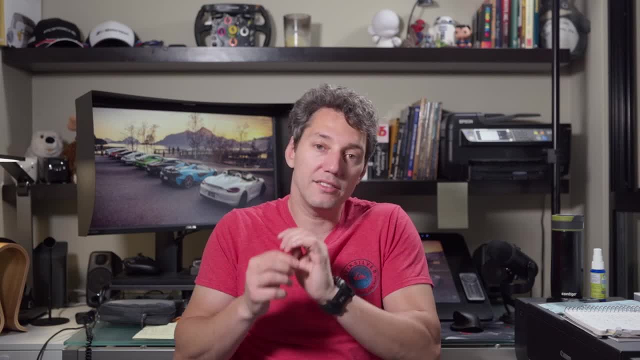 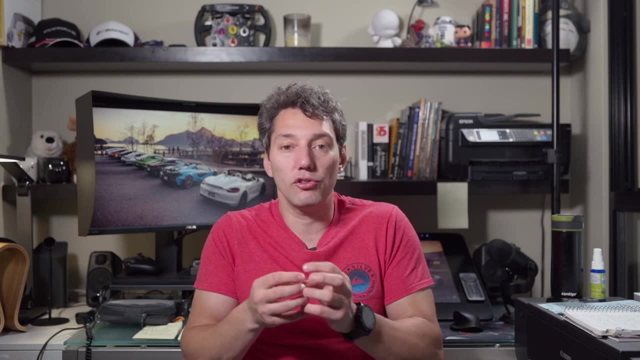 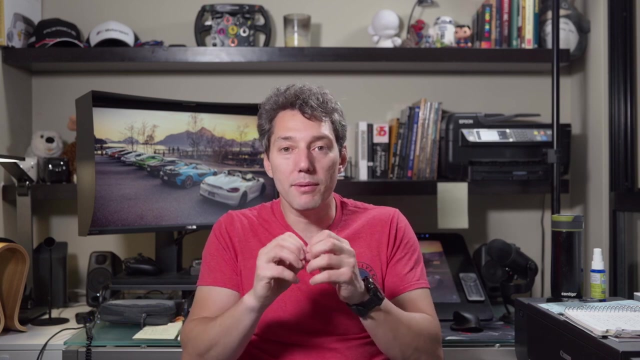 through chemical reactions. now they do not match 100 percent at the original pigments but they are close enough and also because it's a process we can control, we can actually create all sorts of tones and variations of those colors. but if you want to pick the pigment, 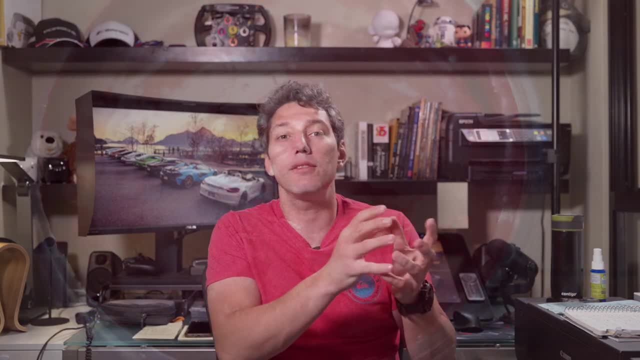 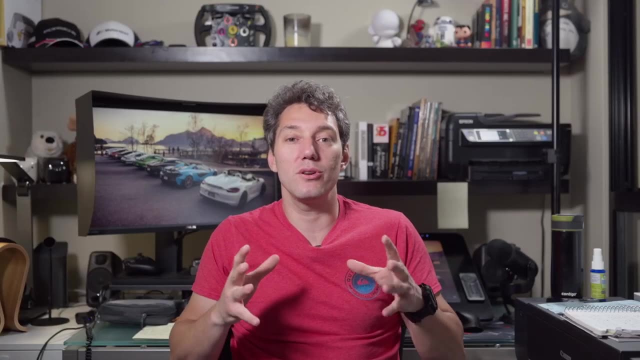 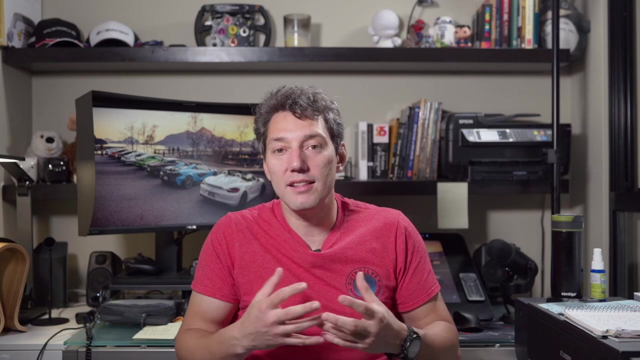 that is actually in nature. for that specific red, for example, like carmine red, you have to buy that pigment, which is going to be really expensive because those pigments are really limited in nature, and that's why we have also come up with the synthetic colors, because 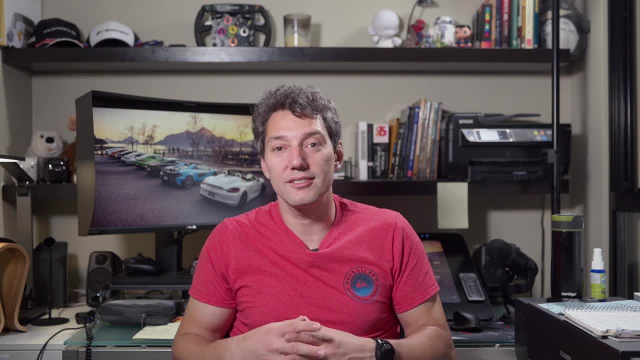 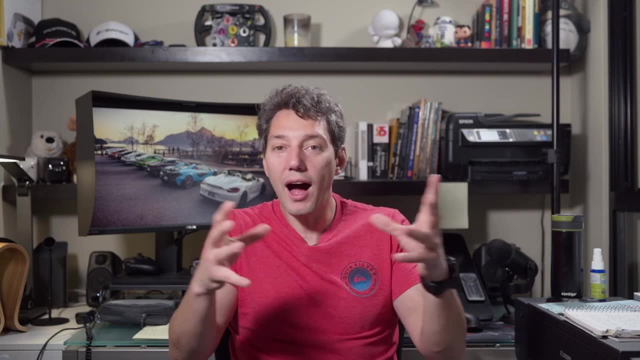 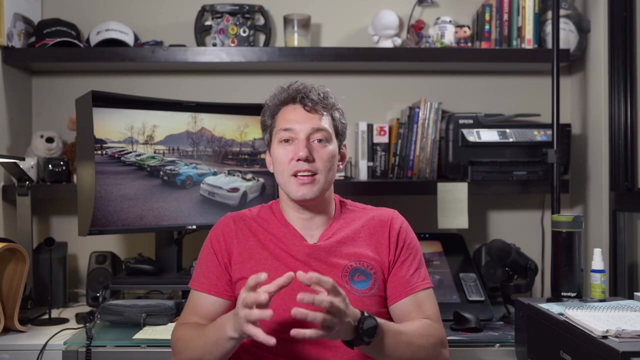 using those pigments gets really expensive really fast. so i hope this was an interesting video. it's a little bit less technical, but it's just to give you an idea of how things around us are made and are colored. in the next video we will talk about the psychology of colors and how the colors affect. 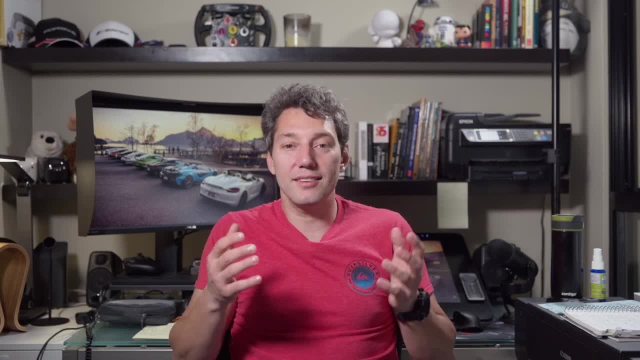 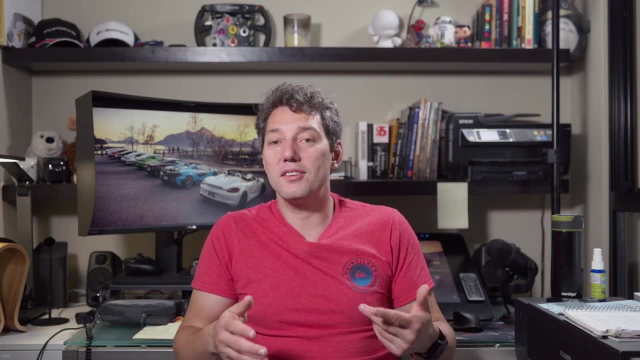 our perception. please, if you like my content, subscribe to my channel and hit the bell so you don't miss any of my new videos. this channel maybe. hit the bell so you are notified of the new videos and feel free to leave a comment below asking me for new topics to talk about. i'm always happy to reply and to read your. 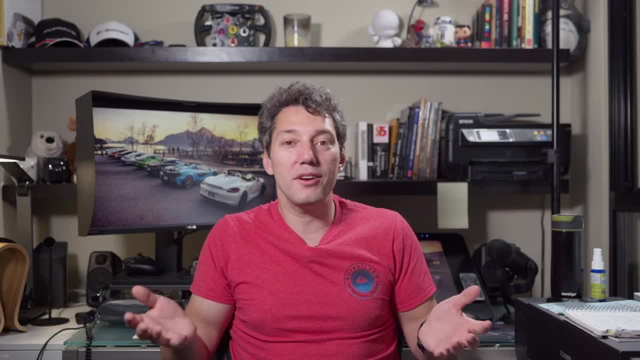 comments and i hope you enjoyed this quick video about colors. that's it for today. i'll see you in the next one. bye.